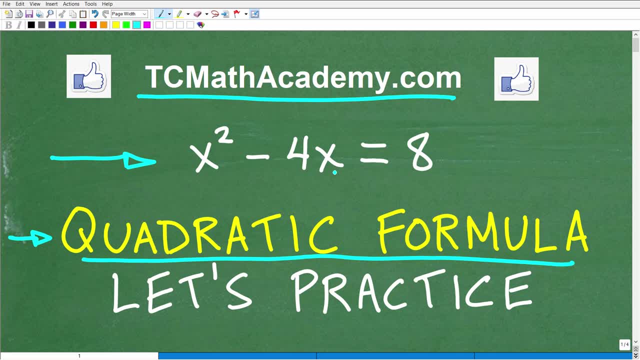 And if you're taking any sort of algebra, this is an absolutely must know concept and skill. Also, if you need math help with the course you're taking, test prep or homeschooling, make sure to check out my math help program at TCMathAcademycom. 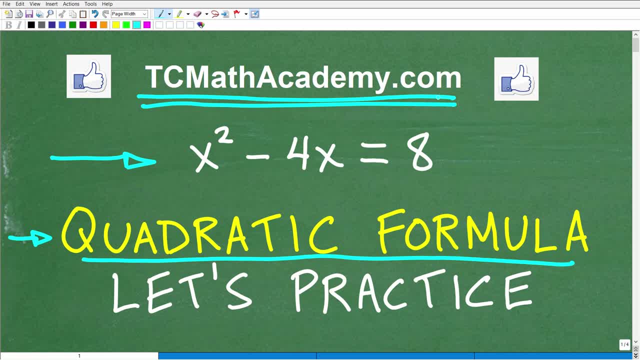 You can find a link to that in the description below, And if this video helps you out, Don't forget to like and subscribe, as that definitely helps me out. OK, so let's go take a look at the answer. here We have x squared minus 4x is equal to 8.. 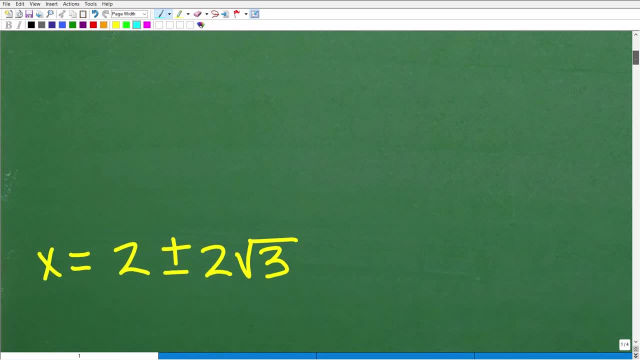 What is the solutions to this quadratic equation? Well, here they are right here. X is equal to 2 plus or minus 2 square root of 3.. So this is what you should have, And this is right. here is actually two solutions. 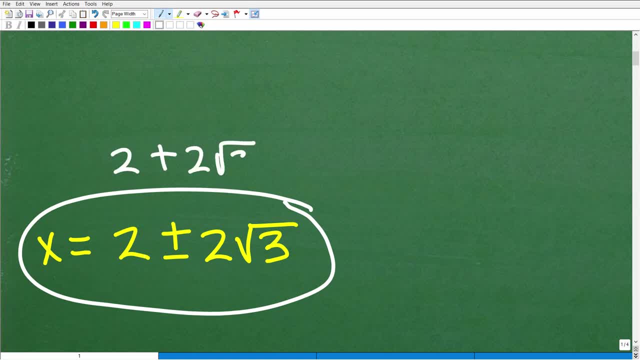 So 1 is 2 plus 2 times the square root of 3.. So this would be one solution And the other solution would be 2 minus 2 times the square root of 3.. But kind of use this shorthand right here, this plus or minus. 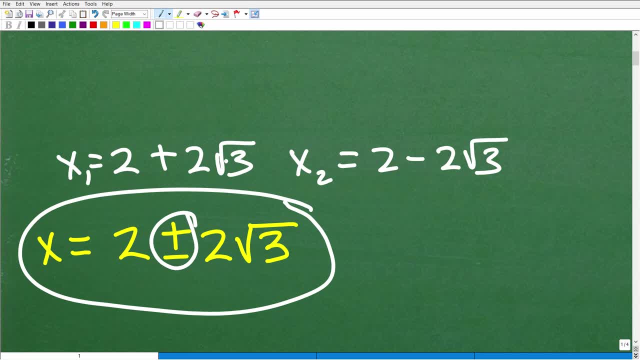 So we don't have to kind of, you know, be a little bit redundant here with writing all this out, So this is the most correct answer. Now, some of you may have gotten pretty close, but you didn't maybe finish simplifying your results. 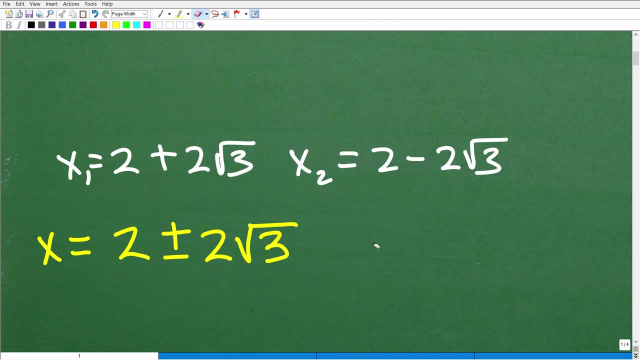 Either way, if you're going to do this particular equation in an algebra class or some sort of math class, this would be considered the most correct answer. Okay, so how'd you do? Well, if you got this right, that is very, very good. 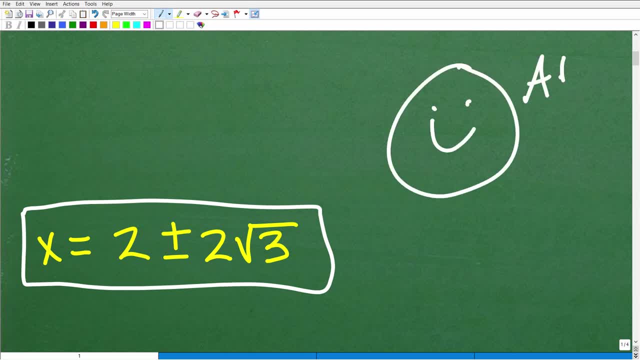 Matter of fact, I'm going to give you a nice little happy face and a plus, plus a 110%, and multiple stars, So you can celebrate your knowledge and skill with the quadratic formula and quadratic equations, Because this particular equation, in fact, you do need to use a quadratic formula. 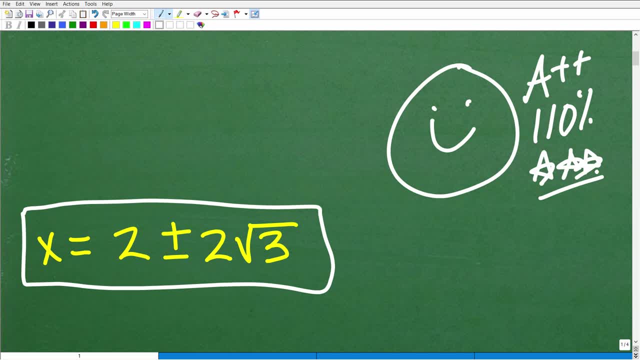 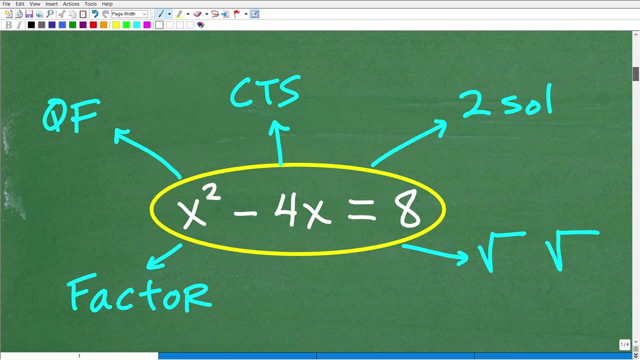 To solve this particular equation. Now, there is some other techniques you can use to solve this, but let's just go ahead and start talking about this right now. Okay, so here is the problem. We have: x squared minus 4x is equal to 8.. 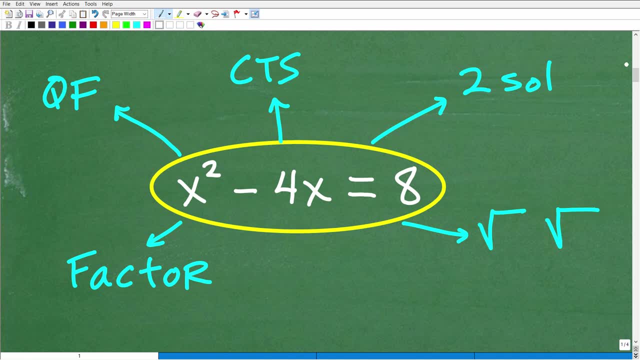 So, of course, I have some things here that you want to be thinking about anytime you are faced with a quadratic equation. So, first of all, what is a quadratic equation? Well, it's what we call a second degree polynomial. So here we have an x squared. 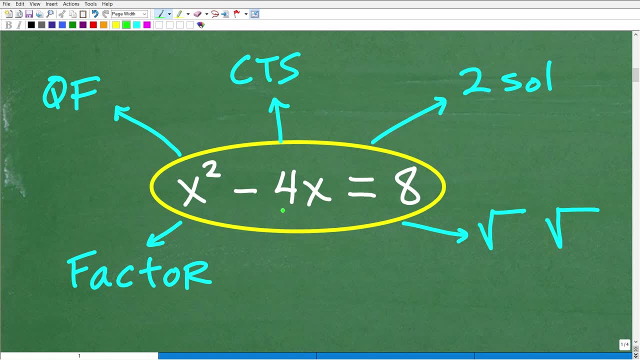 Now, some quadratic equations don't have an x term And of course this variable is y. You know, all these variables are just. you know this would be y squared and this would be 4y. So don't let the x squared, you know, kind of like confuse you. 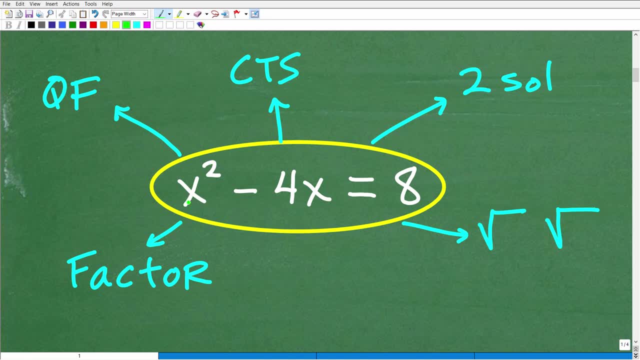 It could be any variable, but any variable squared. We're talking about a polynomial squared where the highest power in the equation is 2.. Okay, So when you recognize you have this type of equation- of course this is an equation- The first thing you need to say is: okay, this is a quadratic equation. 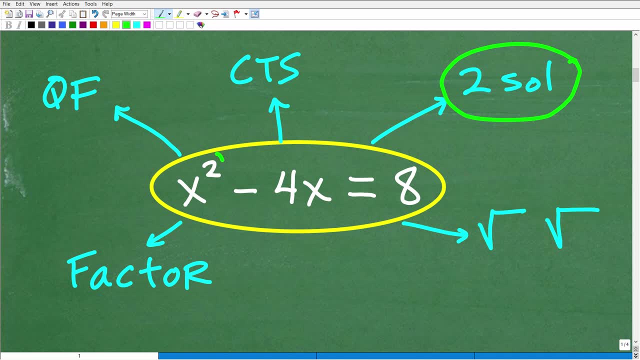 So there will be two solutions. Okay, So this little 2 up here indicates, when you have a polynomial, that you're dealing with a second degree polynomial, And there's something called the fundamental theorem of algebra. It basically says that, listen, whatever the highest power of your polynomial is, 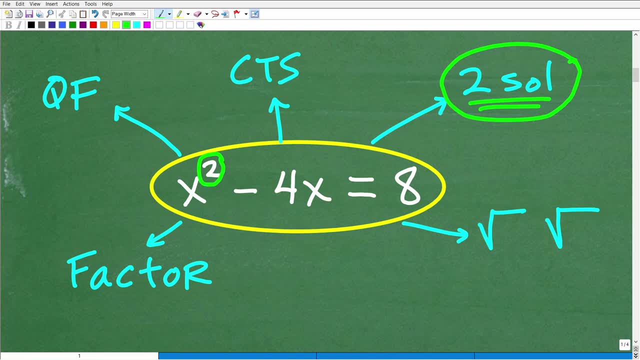 that's how many solutions you're going to have. Now, what type of solutions? Well, here we just don't know that right now We're just kind of looking at the equation. You could have two real number solutions, or you can have complex or imaginary number solutions. 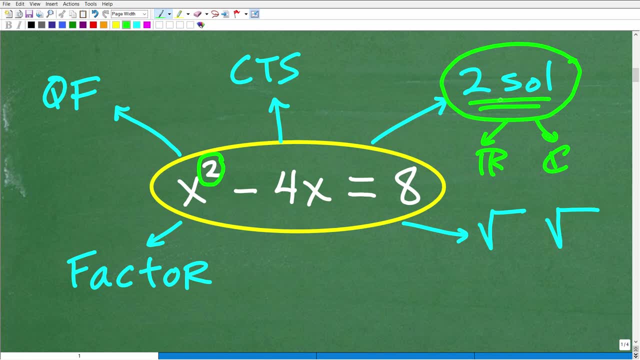 We don't know, but we do know we're going to have two solutions. Okay, so what else do we know about quadratic equations? Well, one method that you need to be aware of is that you could possibly take the square root of both sides. 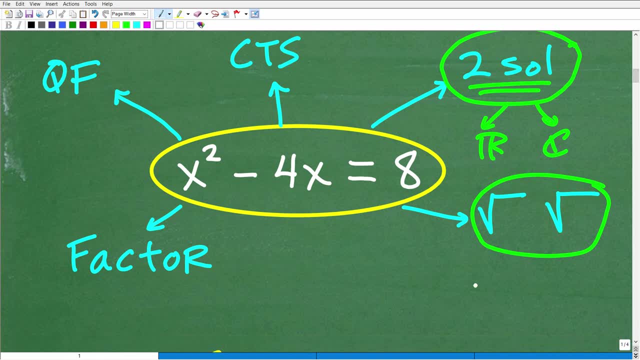 Now that works out when you have a situation where you have a square on either side, Something like x: squared is equal to 16.. You see here this is a quadratic equation, second degree polynomial, but we don't have an x term. 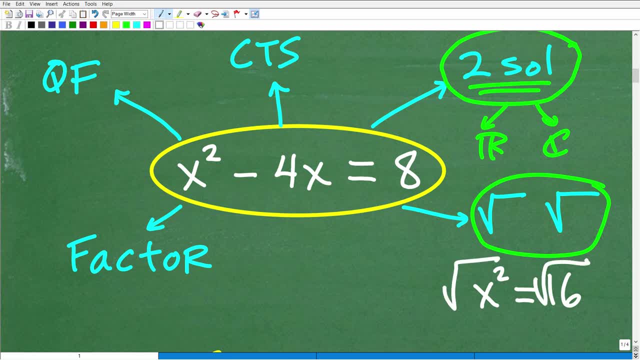 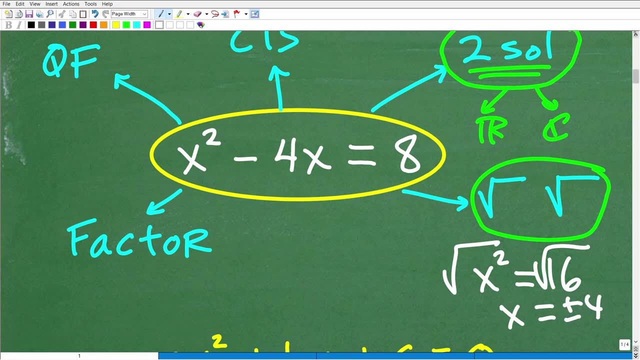 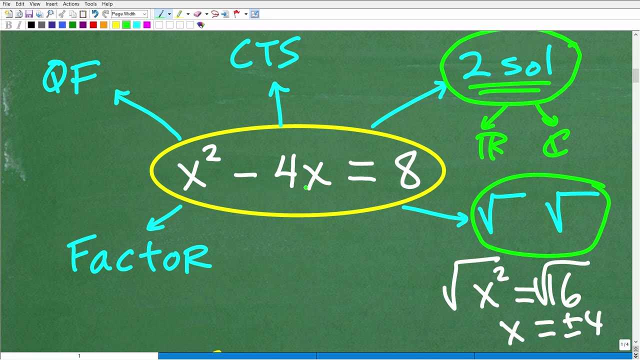 So in these type of situations, we could just simply take the square root of both sides. So this is like super awesome. So x is equal to positive negative 4. That would be the solution to that equation there. All right Now, in this particular case this equation, it has an x term. 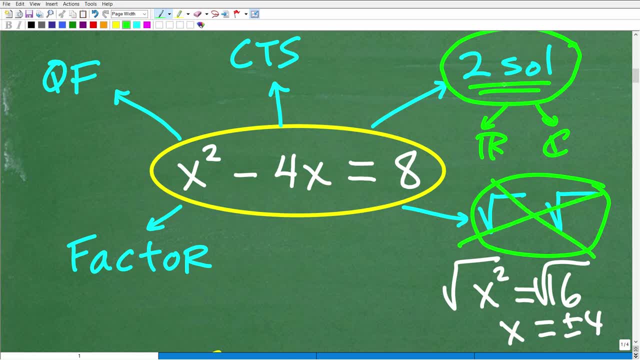 So we're not going to be able to do this right now. So we can't do this. We know this has two solutions. So what we want to kind of look at next is: can we factor this right? In other words, if I move this 8 over on this side, I have a quadratic trinomial x squared minus 4x, minus 8 is equal to 0.. 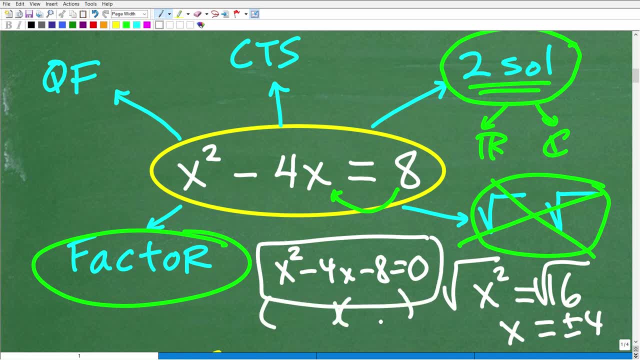 Could I factor this into two binomials? Okay, Now, this is a method that you should attempt to do. Now, you're not going to know whether you could factor this, unless you kind of think about it. Okay, Unless you kind of move this 8 over and you attempt to factor this. 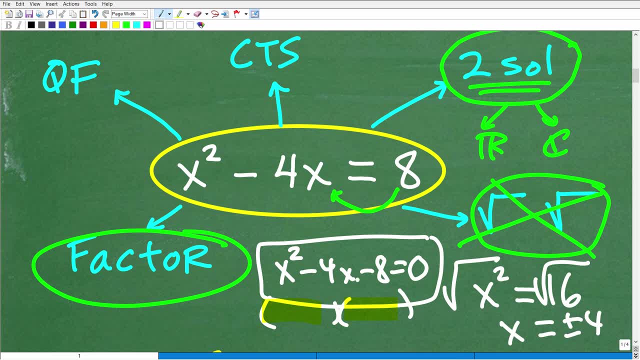 But in this case, this trinomial, you cannot factor this. This is what we call a prime trinomial, So we cannot factor this trinomial. Now, if you could, you kind of want to use factoring, But if you cannot factor and you can't take the square root of both sides, well, what are we left with? 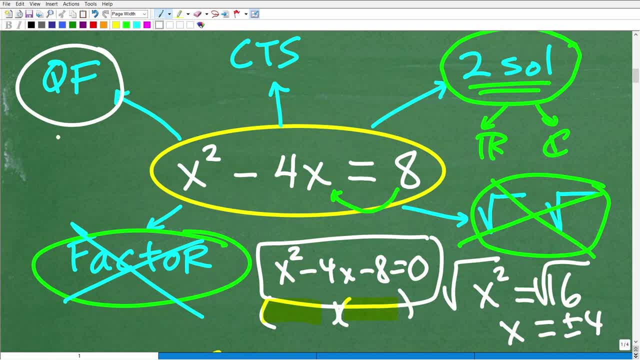 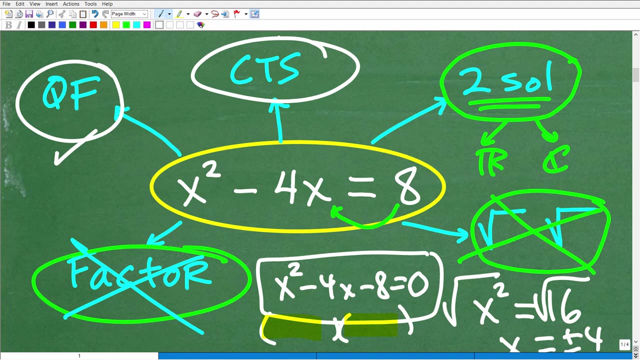 Well, we have the quadratic formula to the rescue. Okay, The quadratic formula will solve any quadratic equation. So anytime you know we can't use any of these other techniques, we can always go to the quadratic formula. And there is another technique called completing the square, which is kind of like the long version of the quadratic formula. 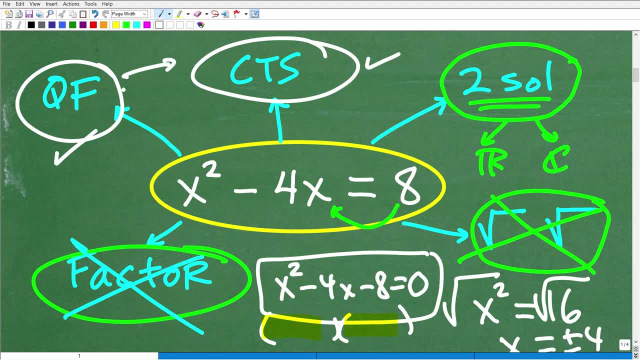 You need to know this as well. But from a practical standpoint, really, if you can't factor, if you can't take the square root of both sides, you're just going to fall back on the quadratic formula. Okay. So in the beginning of this video I kind of stated, said: hey, if you think you can solve this using another technique, go ahead and try. 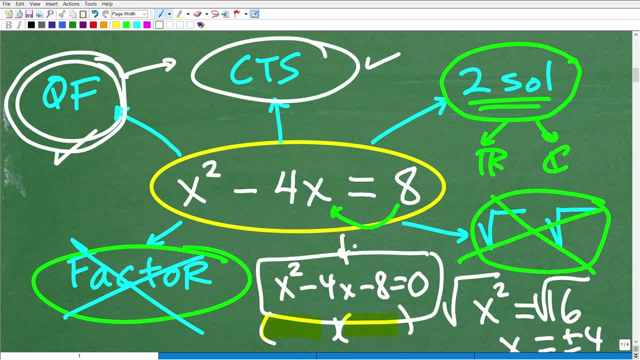 Okay, Probably most of you probably attempted to factor this And hopefully you know, you know how to factor it. Like you know, I can't factor this, So I do have to go to the quadratic formula. Okay, So what is the quadratic formula? 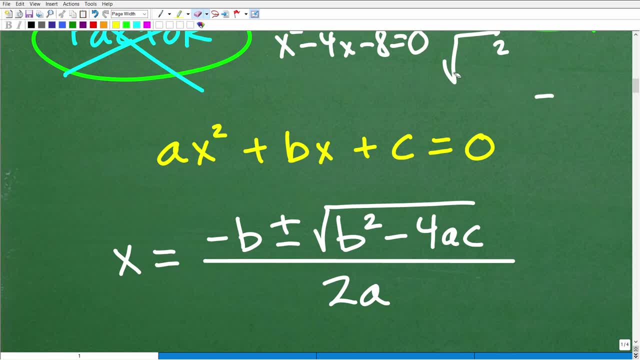 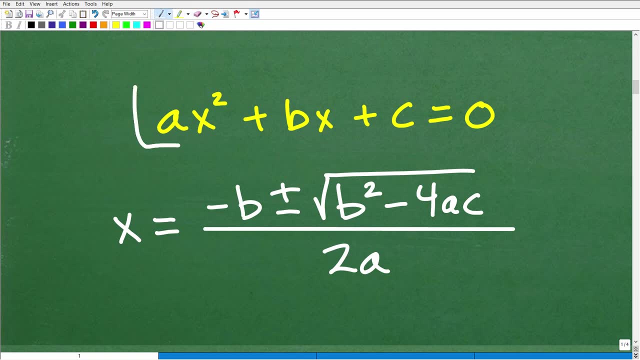 Well, here it is right here. So just in case you forgot what it looks like, this is basically it, All right, So let me explain this here real quick. So here is a quadratic equation in what we call standard form, All right. 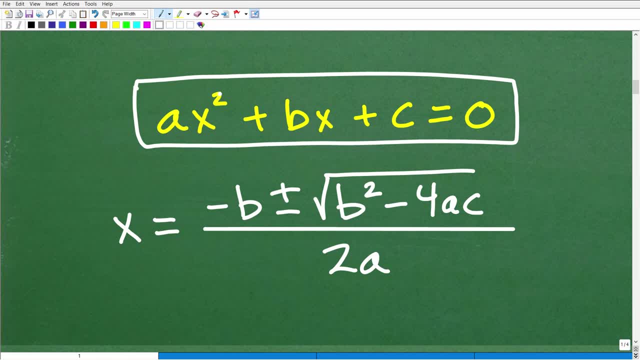 So this is just a general quadratic equation: AX squared plus BX plus C. A is the coefficient here of the X squared term, B is the coefficient, ie these are numbers right in front of these variables, And then C is just a number all by itself. 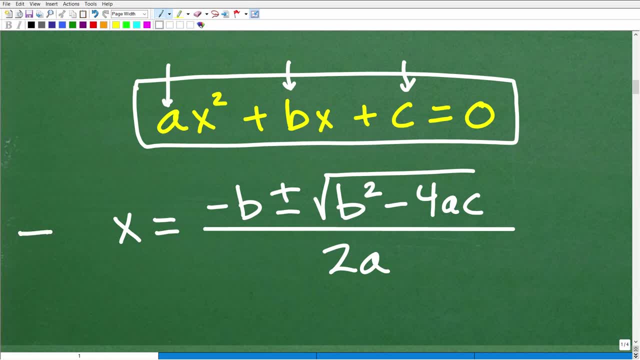 So when we know the A, B and C values, we plug it into the actual quadratic formula, Which is the following: right X is equal to minus B, plus or minus the square root of B, squared minus 4AC, all over 2A. 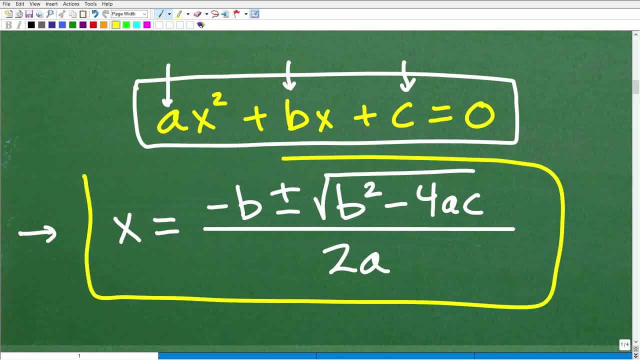 This formula here I would commit to your long-term memory. Now, there are a lot of formulas in algebra and mathematics And that's why you take notes, because you can't possibly memorize all formulas But this one. here I'm going to suggest that you do kind of memorize this. 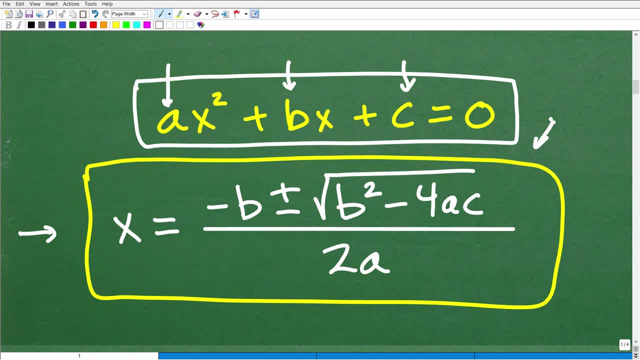 In other words, you know, reference your notes just to make sure you have the correct formula, But as you practice this, try to you know, actually remember this, So you can just kind of draw upon it at any time. Okay, 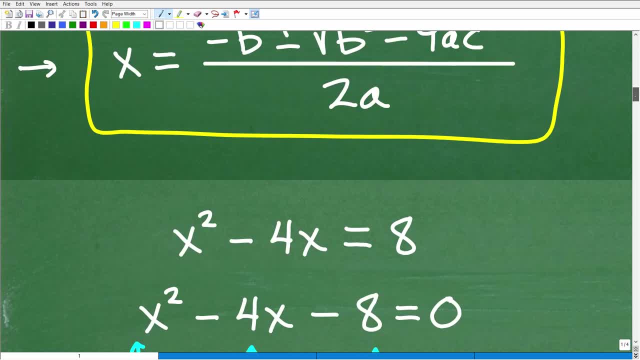 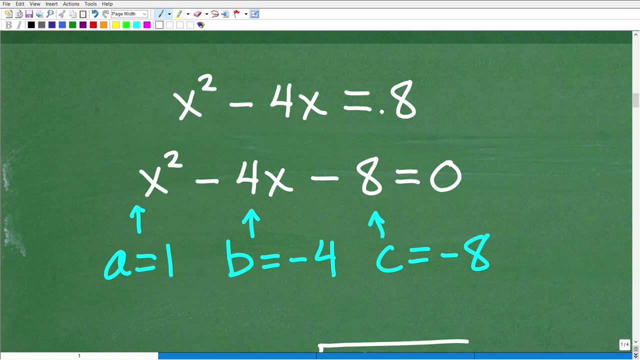 So we're going to be using the quadratic formula to solve this quadratic equation, And let's go down here and take a look at the actual problem. So we have: X squared minus 4X is equal to 8.. Now here this the way the equation is written out. 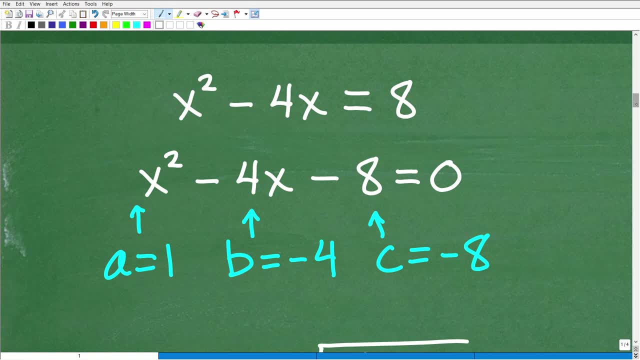 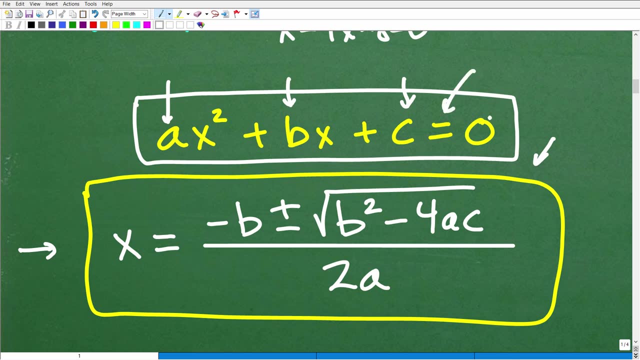 It's like this. It's not in standard form. Okay, Now standard form, In other words, we have to get an equation where everything is on one side of the equation And then we have it equal to 0.. Okay, 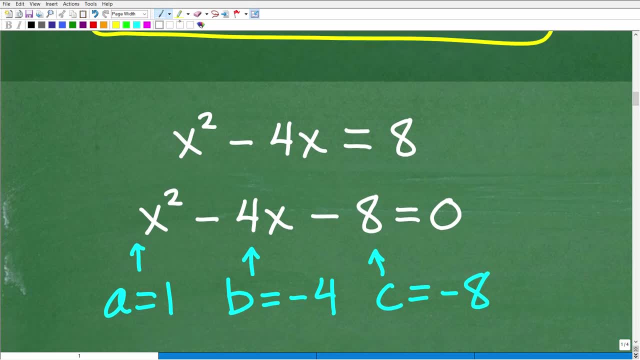 Now here we don't have everything on one side of the equation. We have this 8 on this side, So we're going to have to move this 8 over here. So we'll subtract 8 from both sides of the equation. 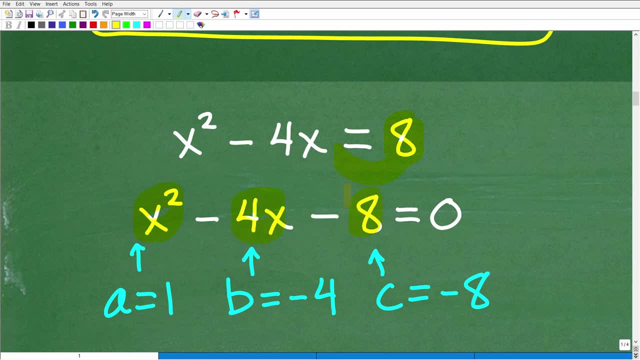 And now we have X squared minus 4X minus 8.. And you're going from highest to lowest power, Right? So you have X squared And then your number. So this is our AX squared plus BX plus C format. Okay, 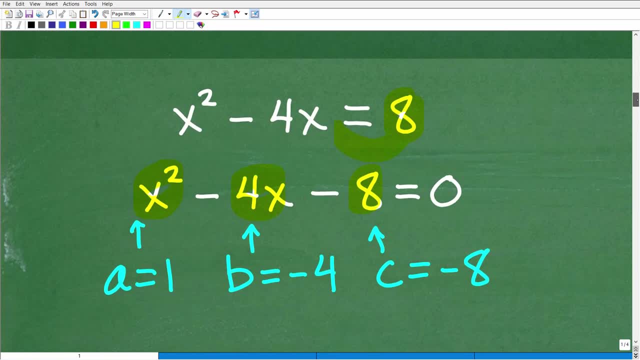 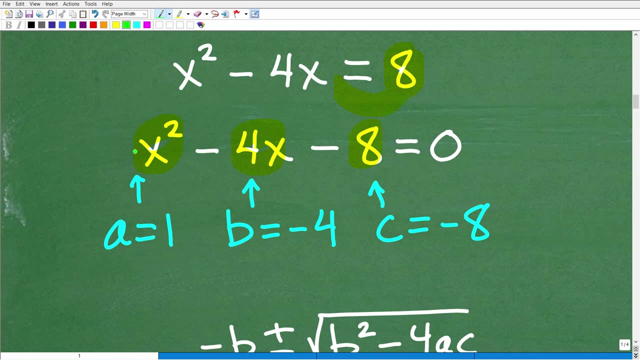 So, in other words, right here, you can see it's in this form, right here, Okay, All right. So at this point, what we can do is go ahead and identify the coefficients, which are the numbers in front of these variable terms. 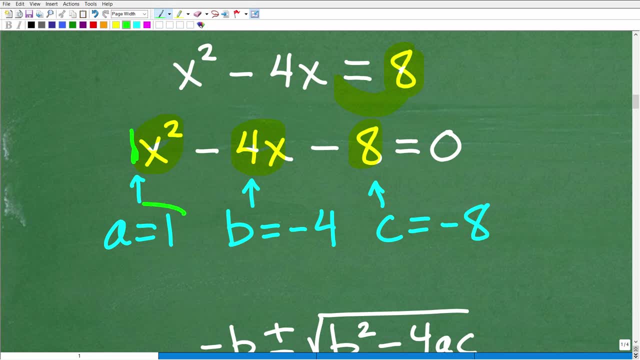 So right here there is a 1.. Okay, And 1 right there, So our A is equal to 1. here There's a negative 4. right here, That's a negative. So our B is going to be equal to negative 4.. 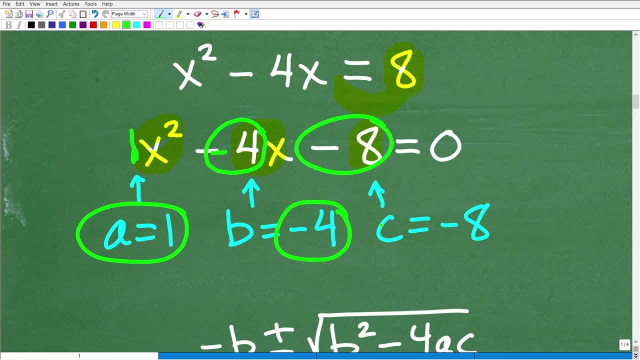 And then our constant here is negative 8. So that's going to be our C value. So we have our A, B and C values. So I've kind of set all this up for you. So if you're like, okay, I understand. 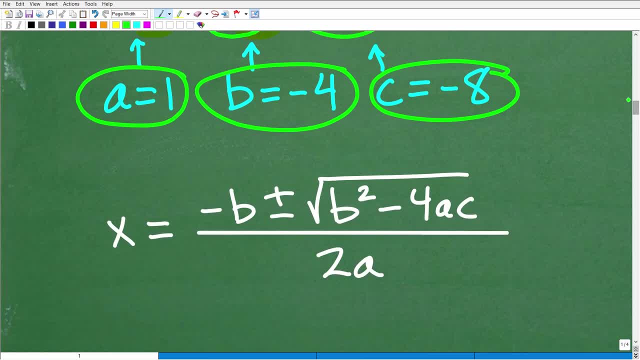 Well, that's great, Okay, So if you didn't get this problem right, go ahead and plug in these respective values for A, B and C into the quadratic formula And then simplify this thing and see if you can get the right answer, which I kind of 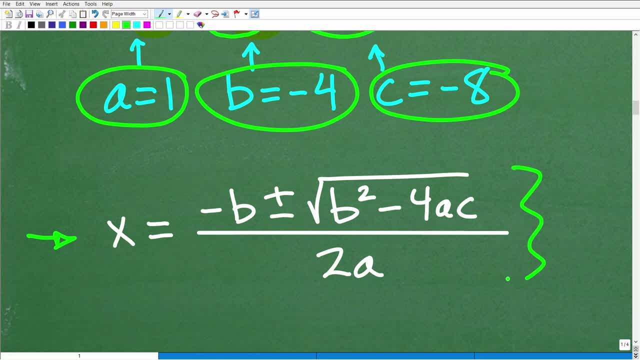 showed you in the beginning of this video, Because this just kind of doing the math here gives a lot of students trouble, Okay. So I want to give you an opportunity to practice this if you were kind of confused in the beginning of this video or the problem you weren't quite sure what to do. 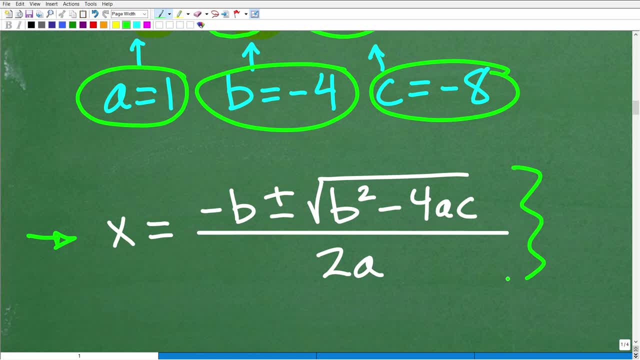 So see if you can do this part, because if you can't do this part, then obviously you're going to need to be able to practice using a formula, which is this In the whole idea of this video. All right, So let's go ahead and do this right now. 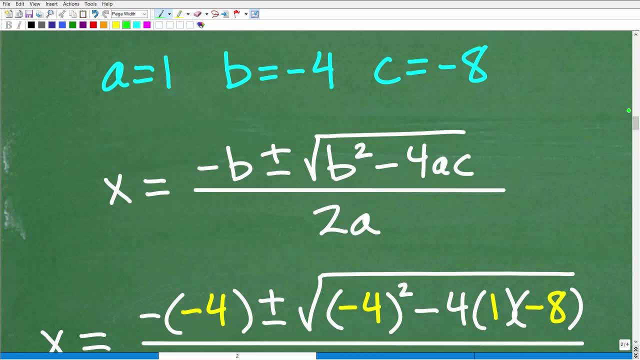 Okay, So here we have our A, B and C values. So here's the quadratic formula. So we're going to have to be super careful to replace each one of these variables with these values. So here's B, So we have minus B, So I have to replace this B with a negative four. 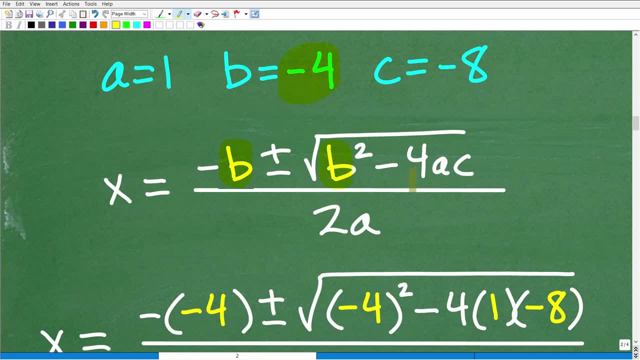 I'm also going to have to replace this B with the negative four. And then of course I have A- I don't have to replace that with one. And then C- I'll have to replace that with negative eight. And then here A is with one. 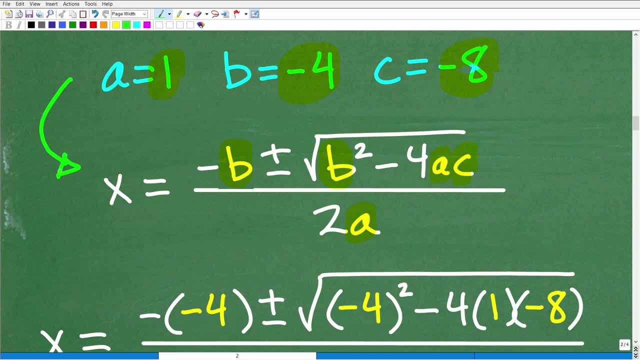 Now, when you're plugging your values into the quadratic formula, you want to use parentheses. Okay, So in other words, here I have minus B, Use parentheses to plug in your values. So this B is negative four. So you're going to have a negative parentheses, negative four. 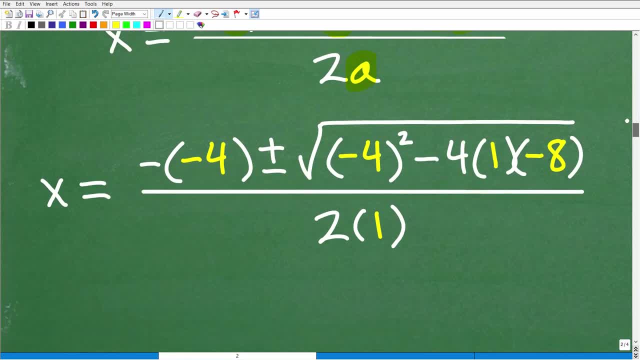 All right. So let me show you all this work right here. So this is minus B, So it's negative, It's a square root of a negative four plus or minus square root. parentheses again right. Negative four squared minus four: A, C all over two A. 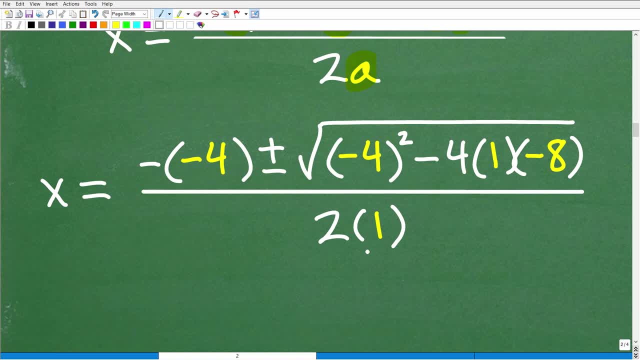 So the first kind of part of using a quadratic formula, after you kind of identified your correct A, B and C values, is to be super, super careful plugging in those values into the quadratic formula. Now, a lot of students make mistakes. They'll plug in a number. 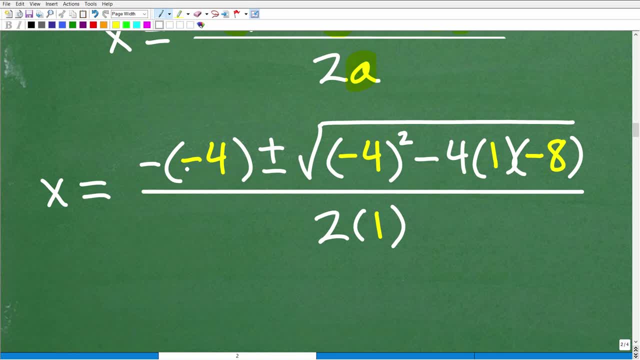 They'll have the wrong signs And if you use parentheses that can really help kind of reduce errors. So before you start doing the math here, double and triple check, You know, go back and say, okay, did I plug everything in correct? 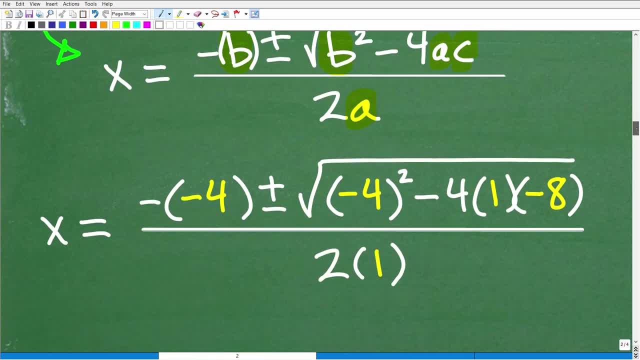 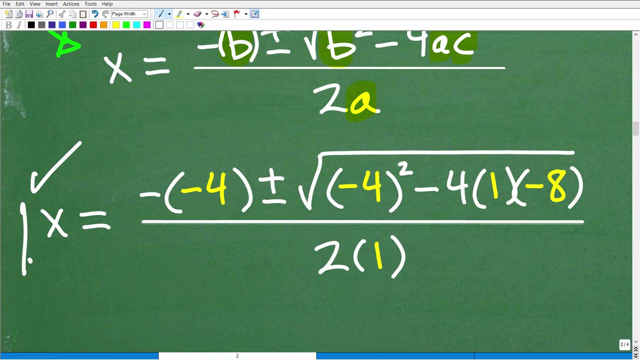 Do. I got my correct A, B and C values, Double check, triple check, And then, if you're like, satisfied that, yes, indeed, you plugged everything in correctly, then from this point forward we can kind of start simplifying all of this. 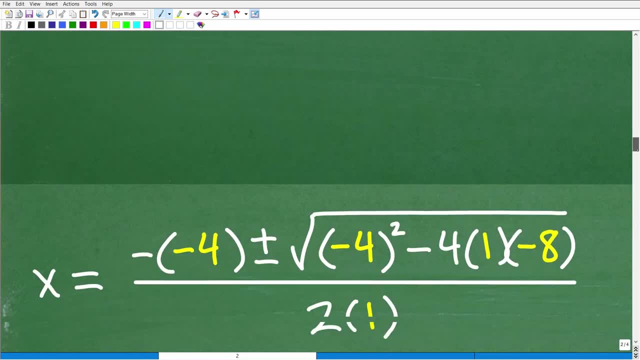 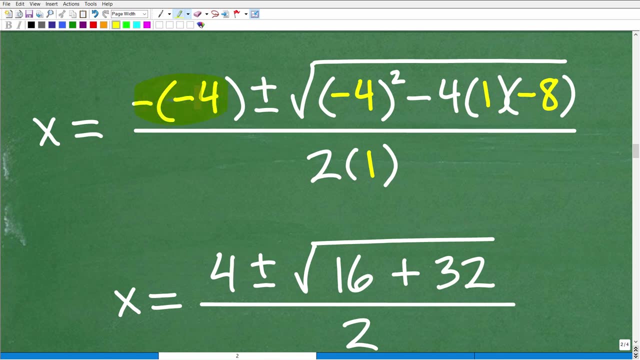 So let's go ahead and get into this right now, Okay. So, first things first. We'll go up here. We have minus on minus four. Okay, Well, of course, opposite of a negative four, That'll be a positive four plus or minus. 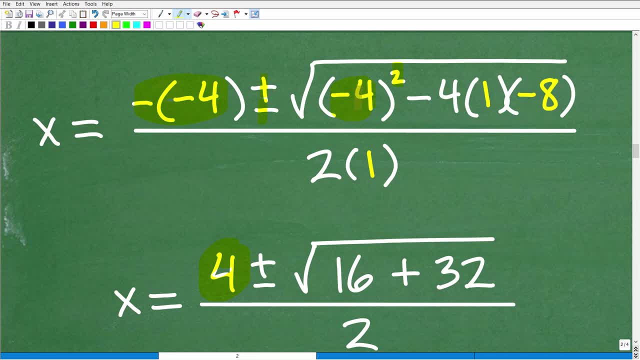 So here is negative four squared Negative four times negative, four is positive 16. Now this part right here, all underneath this square root, is what we call the discriminant, And this is a kind of common error where a lot of students make mistakes with the quadratic. 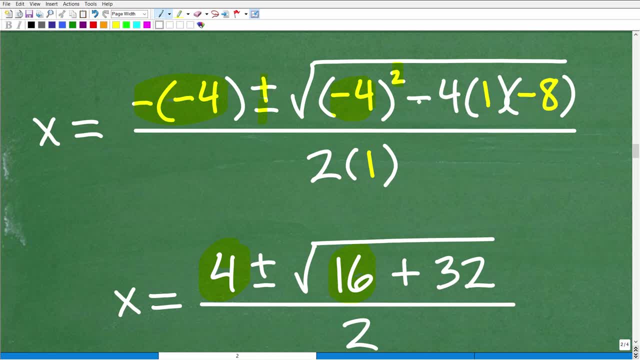 formula. So this minus four, A C part, this minus, if you turn this into a positive four, you'll get a plus negative. That will help kind of identify what sign this number will be. So we have a negative times, a positive, times a negative. 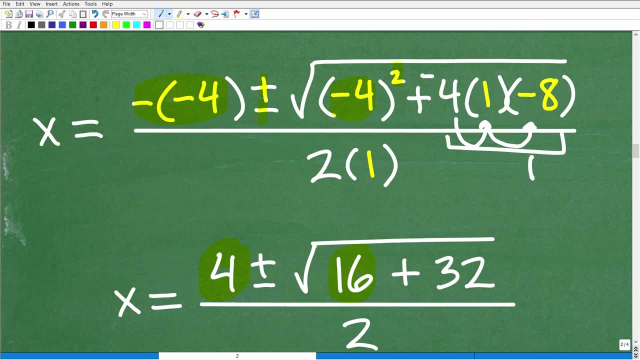 So this is all going to end up being a positive value. All right, So we know that four times, one times negative or times eight is just going to be. we kind of just forget the signs here because we know the final answer is going to be positive. 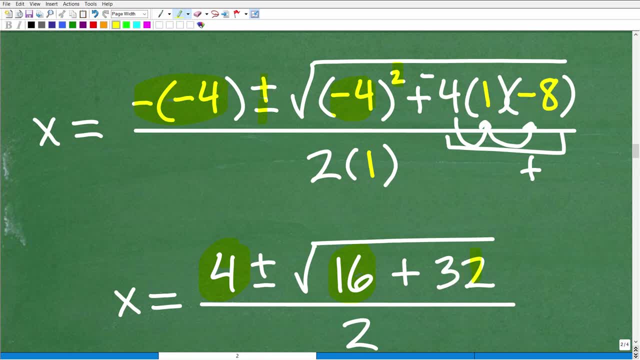 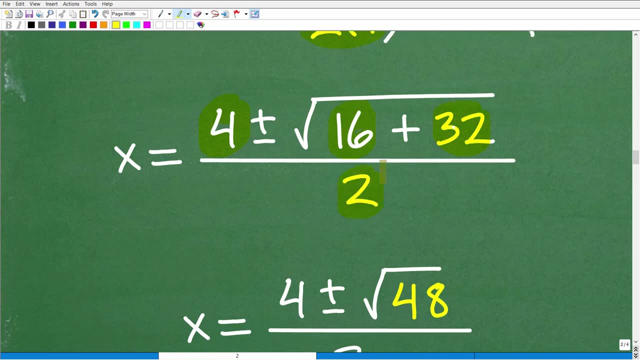 So we just go four times one times eight, which of course is going to be 32.. All over two times one, which of course is two. All right, So you're just going to be working, you know, all this math down step by step. 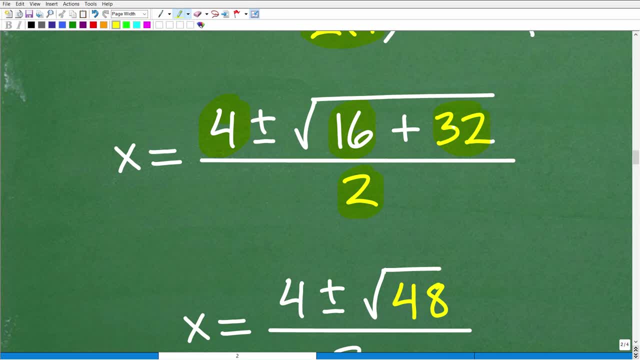 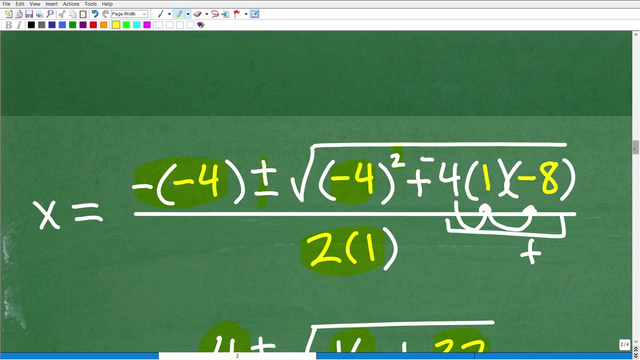 You don't want to take too many steps, You know just. in other words, you don't want to go from all of this, do everything all at once and then have one final thing. You want to take only one or two steps and continue to write. 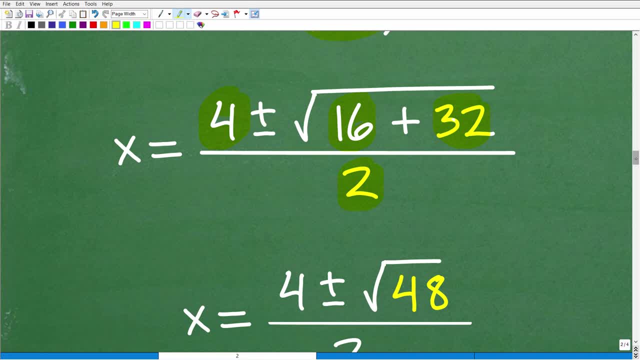 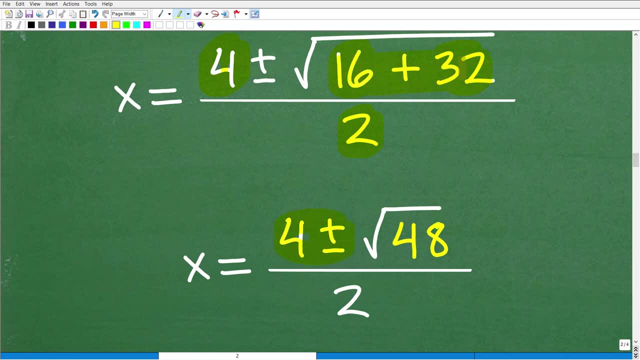 So you and your teacher can keep track of what's going on. All right, So let's go ahead and continue the problem. So we have four plus or minus, Right? So now we're going to add these numbers underneath the square root. 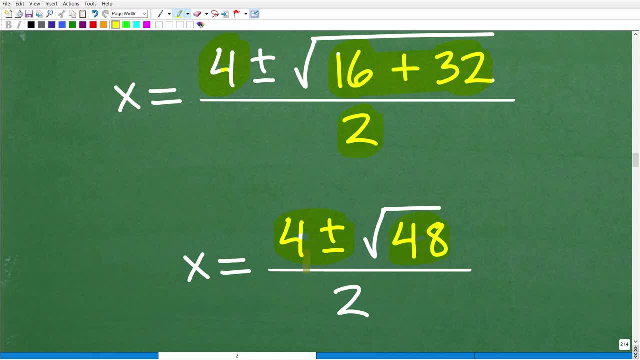 16 plus 32 is 48. So we have four plus minus square root of 48, all over two. Now, if you had this as your answer, I would give you a happy face. Okay, I might even give you an A minus, maybe like a 93%. 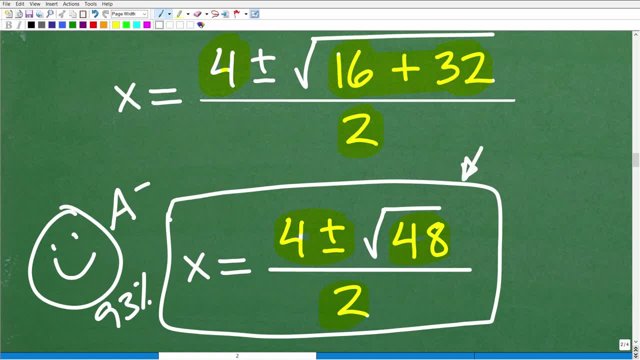 So that's pretty good. But here's the problem: You have some work to do here. This is not fully simplified, But this is, you know, an indication that you did plug in the correct values into the quadratic formula. You know what you're doing, but you're not done yet. 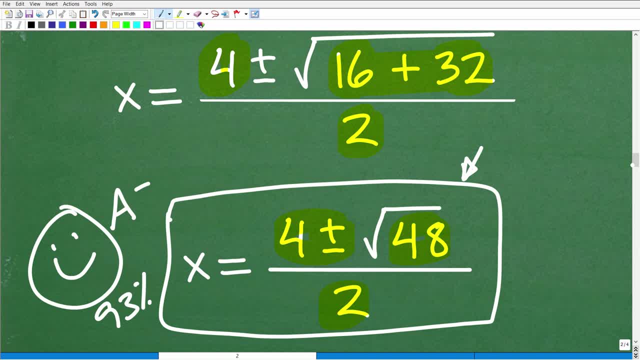 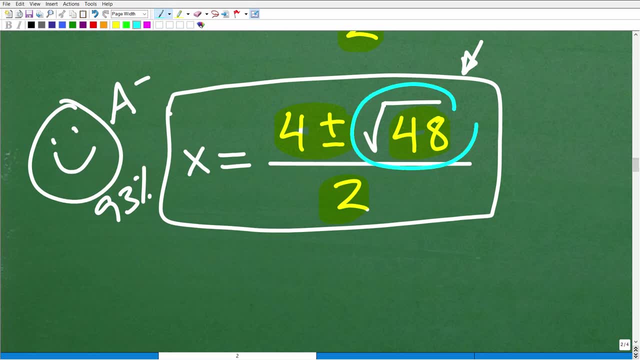 We actually got a decent amount of work to go. So let's go to continue to simplify this situation, And namely, I have this square root, the square root of 48.. Anytime you have the square root when you're dealing with the quadratic equation, you need. 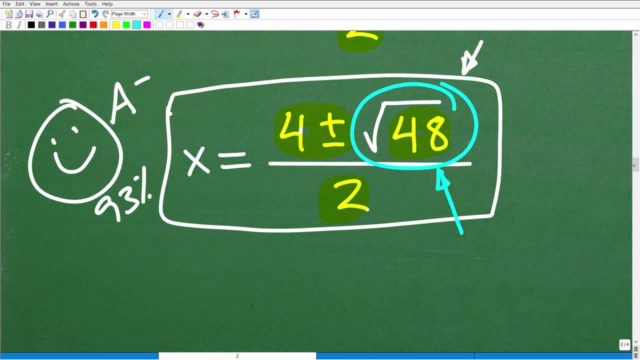 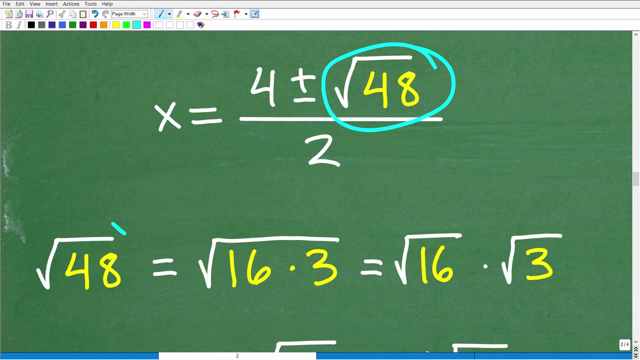 to see if you can simplify this radical, And in this particular case we can. All right, So let's focus in on the square root of 48.. So the square root of 48 is equal to the square root of 16 times three. 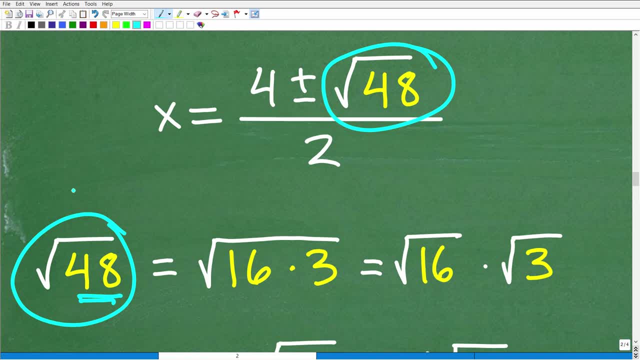 Okay, So you want to look for perfect square factors here? Now, this is a whole nother kind of conversation or skill set, working with radicals and square roots, And at this stage, if you are completely kind of overwhelmed, let me give you a couple of. 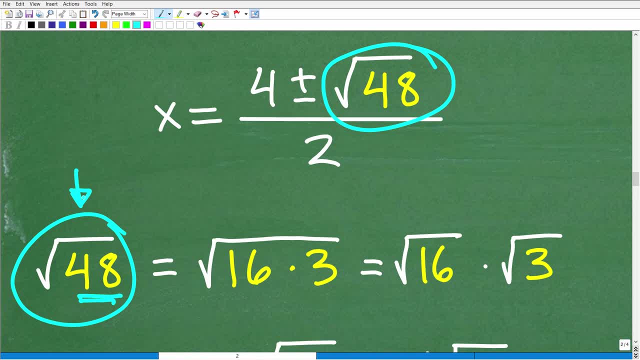 suggestions. One: I'm going to direct you towards my Algebra 1 course and my Math Help program. Also, I have a ton of additional videos. So I have a ton of additional videos on my YouTube channel as well, But make note of what you're not understanding. 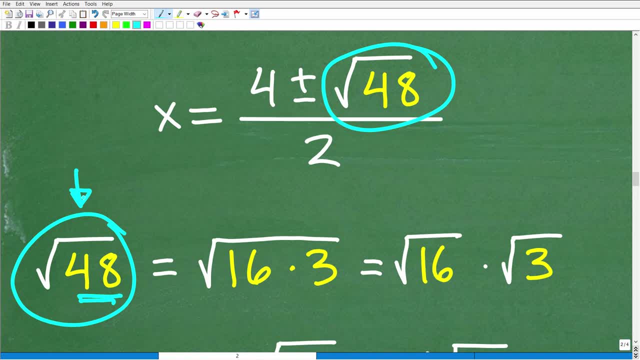 Okay, Because the same thing is going to come up over and over again when you're doing these problems. All right, So the square root of 48, we're looking for perfect square factors. So 48 is the same thing as 16 times three. 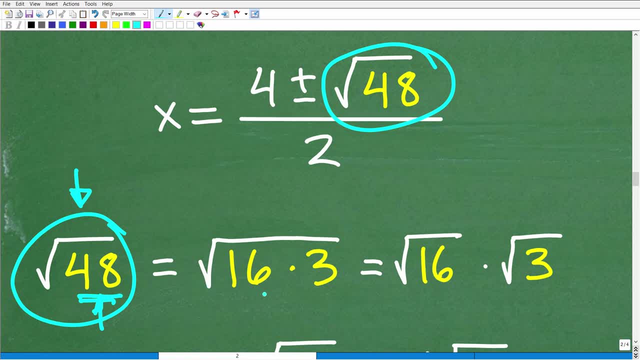 So the square root of 48 is the same thing as the square root of 16 times three, And then I could break this big square root into two separate square roots. This would be the square root of 16 times the square root of three. 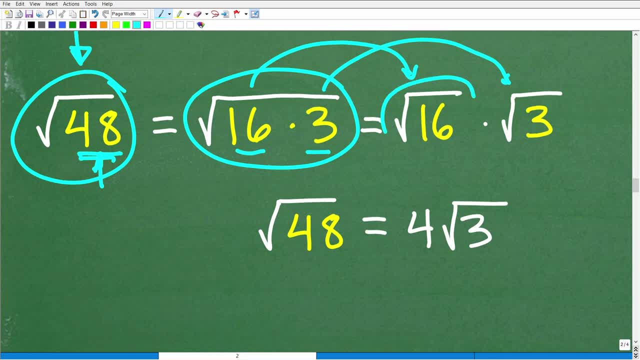 That is a property of radicals, or property of square roots. And now that we have a perfect square factor of 16, we can take the square root of 16, which of course is four. So now we have four times the square root of three. 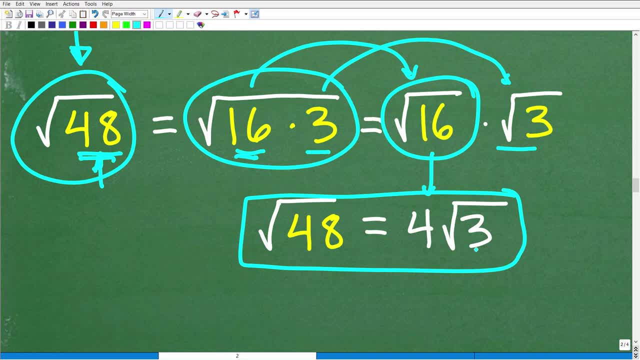 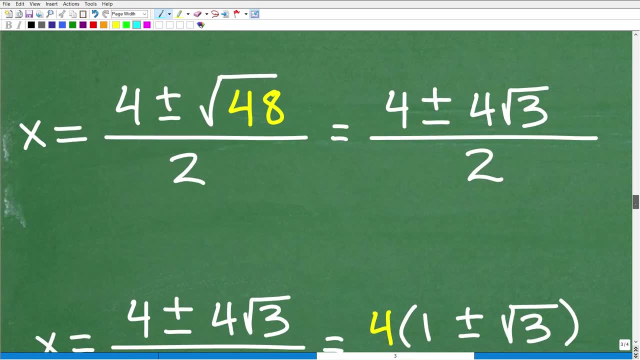 So the square root of 48 is equivalent to four times the square root of three, And that is what we need to use to continue to simplify this problem. Okay, So here is where we kind of left off. We had four plus the square root of 48, all over two. 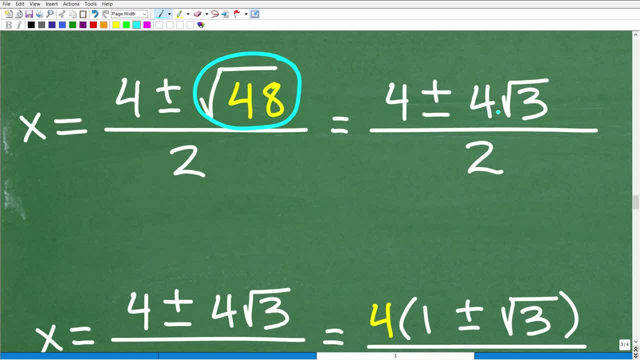 So we did all this work to simplify the square root of 48 into four, square root of three. So now we need to kind of factor out some numbers here, some greatest common factors, and clean this up, because you can see, two will go into both these fours right here. 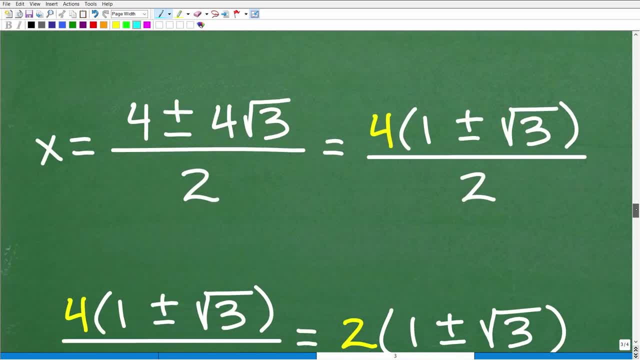 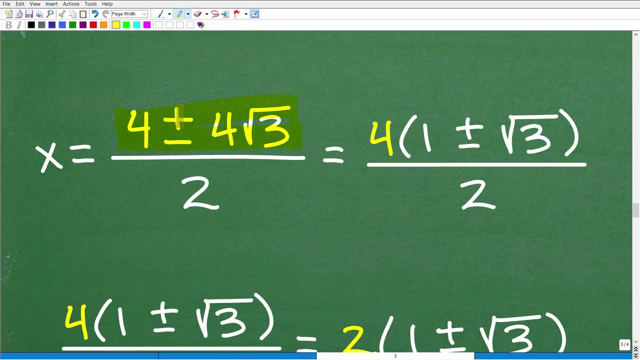 But just to make it super clear on how to kind of simplify this, let's take a look at the numerator here. So here I have a four, And I have a four here, And this is plus or minus. So I can factor out this greatest common factor: four right. 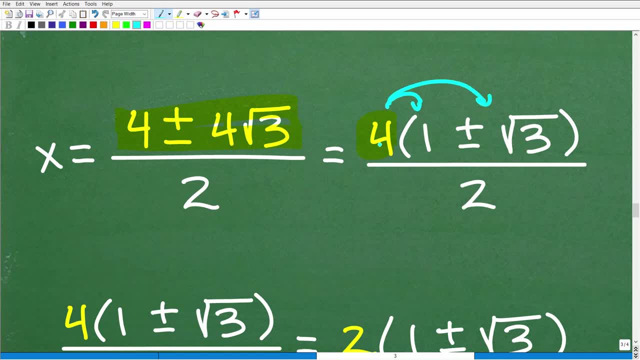 So in other words, if I take that four and I multiply back in, that would be four times one or four. And then this four times that square root of three would be four square root of three. So this is a factor. So now I have two down in my denominator. 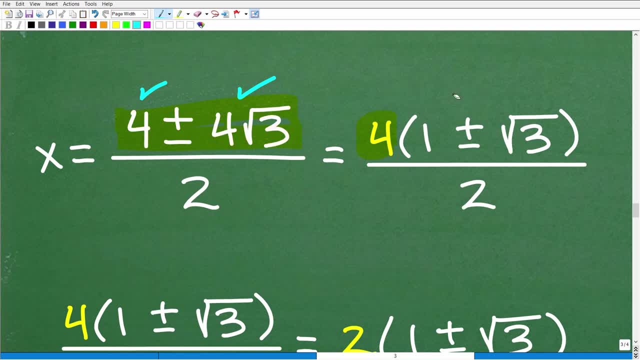 So four of course is the same thing as two times two. So I can cross cancel one, two And that will leave me with a two right there, OK, up in the numerator. So I'll take this two. That will go into that four twice. 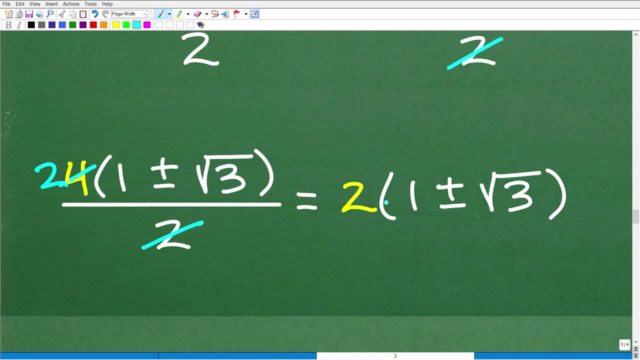 So now I have two times one plus or minus the square root of three, And then, of course, I can distribute back in. take this two and multiply it back in to both of these terms right here, And let's go ahead and wrap this up. 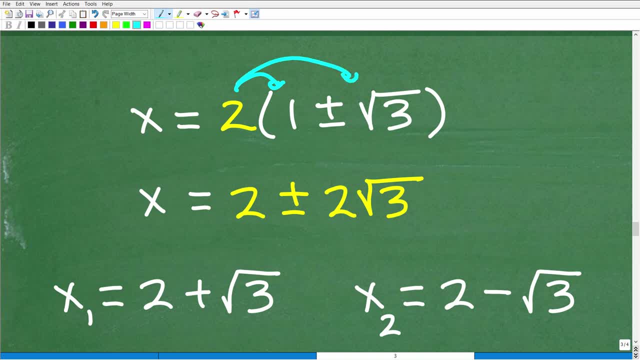 So this would be two times one, which of course is two, and two times the square root of three. So this is the final answer. OK, so x is equal to two plus or minus two times the square root of three.